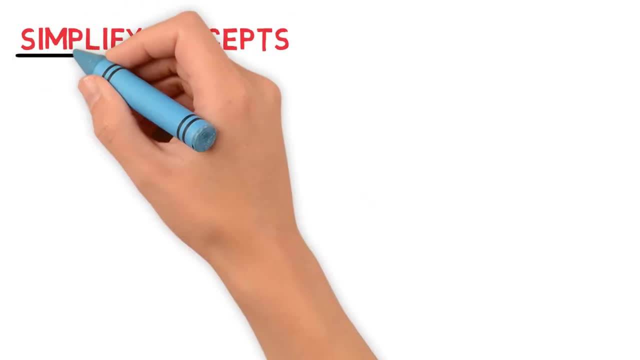 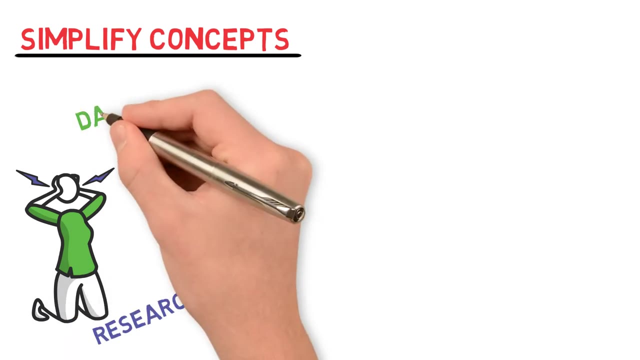 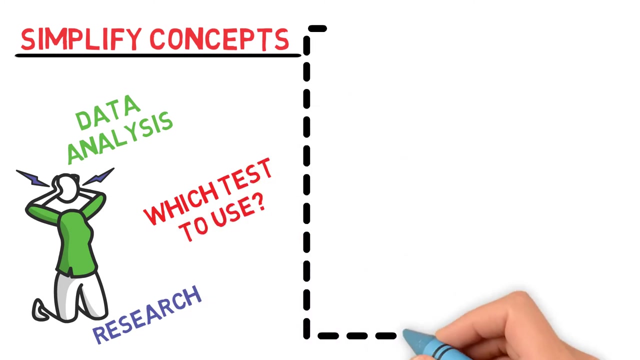 Hi, this is Simplify Concepts and I am Dr Shuchi and we'll be talking about research and related issues like which tests to apply. in this video, So many of you must have collected the data and while doing data analysis, you must have been stuck here: that which test to use? So this: 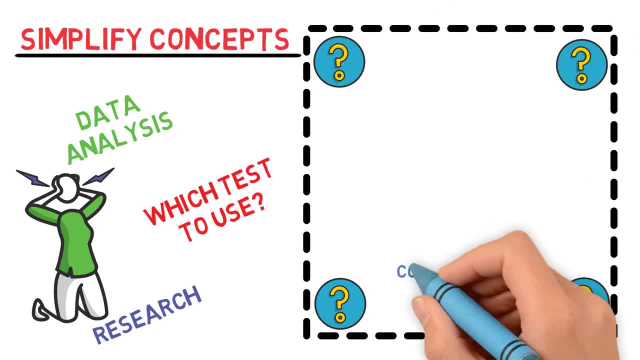 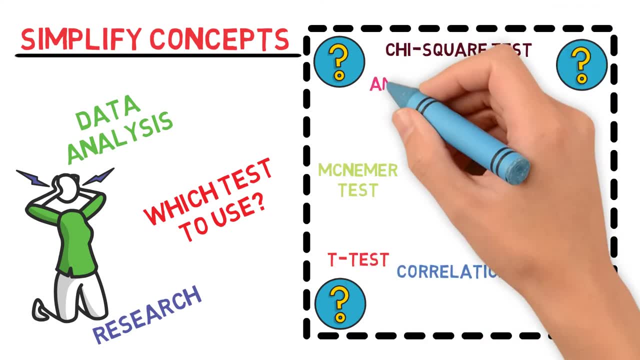 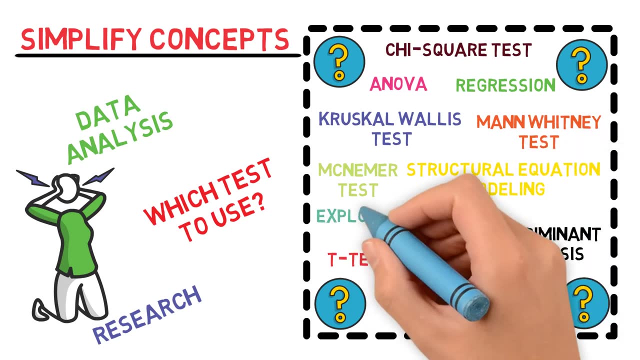 is the biggest question in the mind of every researcher or analyst: whether you should go for correlation or t-test, when to apply discriminant analysis, McNemar test, chi-square test and lot many. So in this video we'll be talking about the different factors which will help us in. 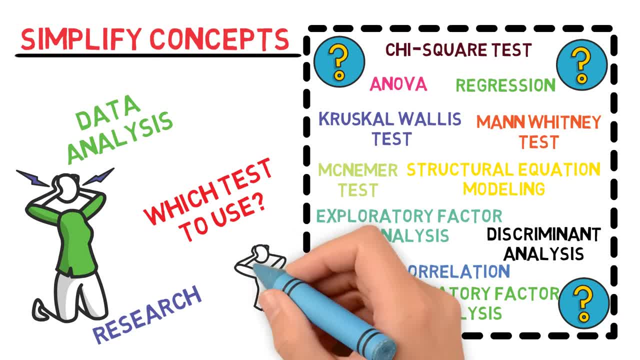 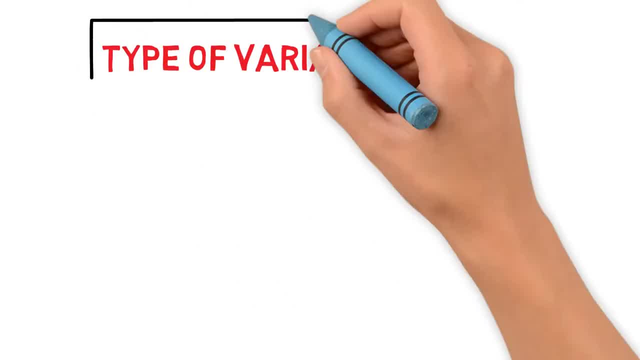 deciding that which test and analysis to use in which situation. So we'll be telling you five such factors here in the video. So we start with the first factor. The first factor is the type of variable. So when you collect the data, then you have different kinds of variables. It may be: 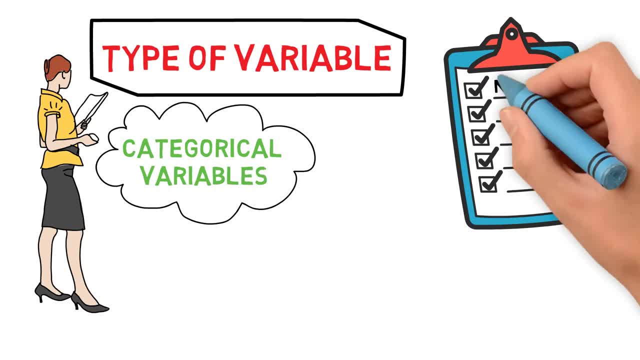 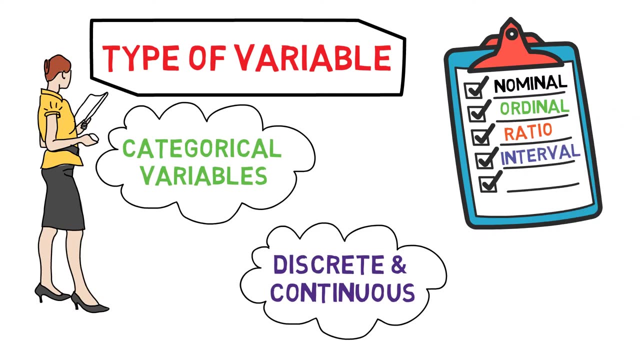 categorical variables. It may be categorical variables. It may be categorical variables, variables which can be measured on nominal scale or ordinal scale. nominal is when you have groups, ordinal is when you have groups which can be ranked. then we can have discrete or continuous variables which can be measured on ratio or interval scale, like you can have the height. 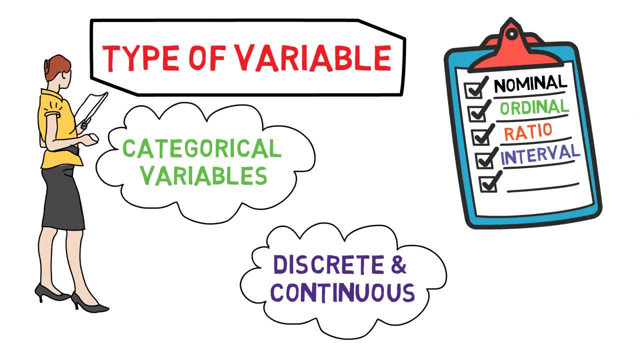 weight. so all these are your continuous variables. then, oh see, meet him. he's our mr Polu and he's a very active listener for all our videos. and see, I think he wants to say something. what happened, Bolu? please give an example. okay, so here's an example for you both. so one of my student, a few. 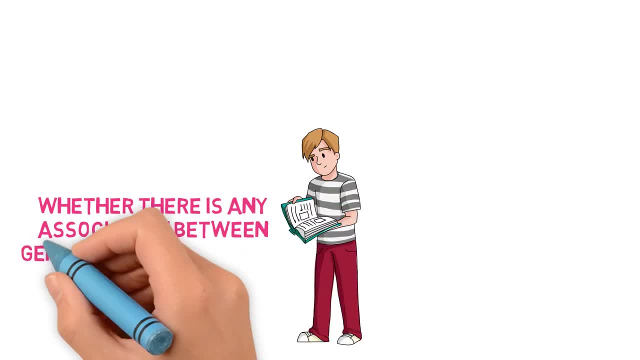 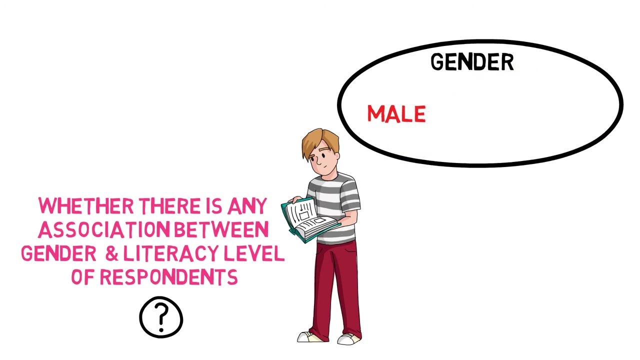 days back he approached me with the question that whether there is any association between gender and literacy level of the respondents. actually has collected all his data, so I told him to tell me more about the variables. he told me that gender has been divided into two categories: male and female, and the second variable, that is, literacy level. again, 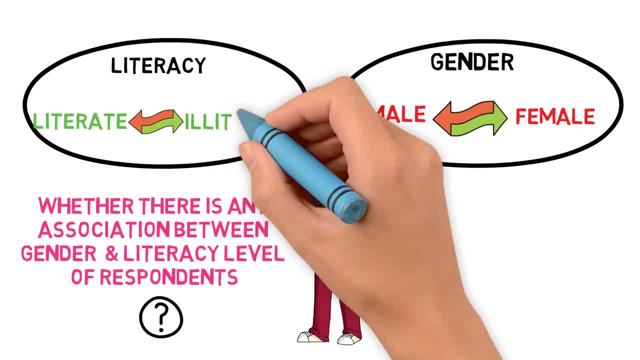 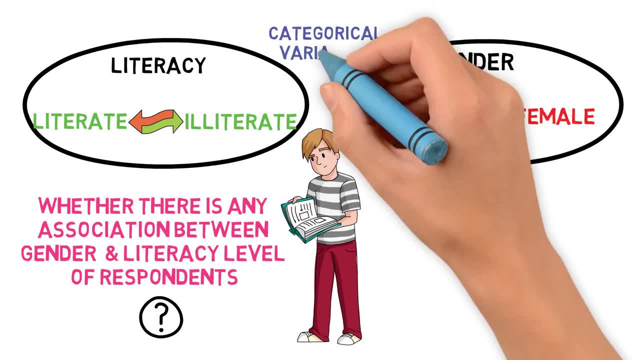 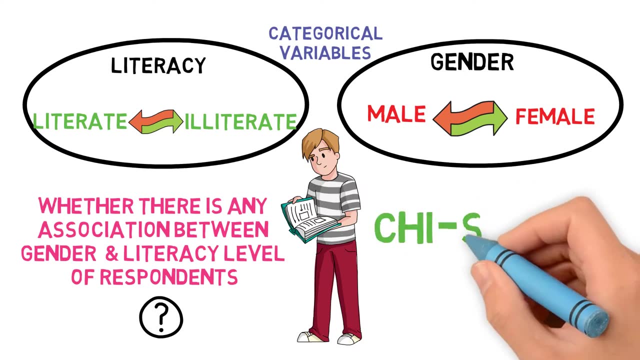 it is bifurcated into two categories, that is, literate and illiterate. so then I told him that these two variables are your categorical variables, and whenever you want to establish your relationship or study the relationship between the categorical variables, the best way is that you can apply the 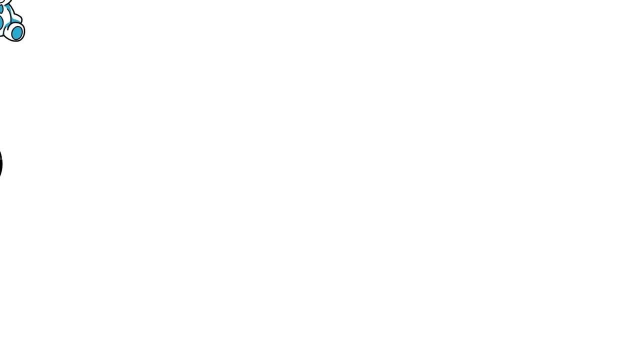 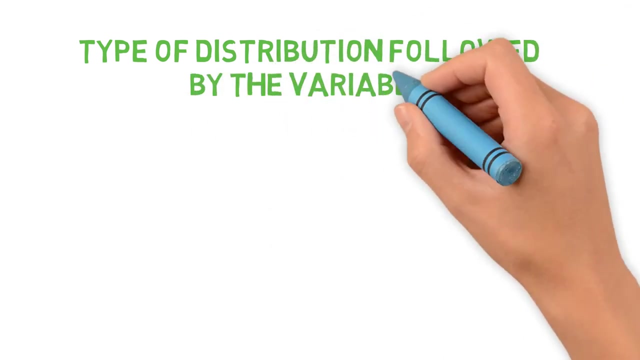 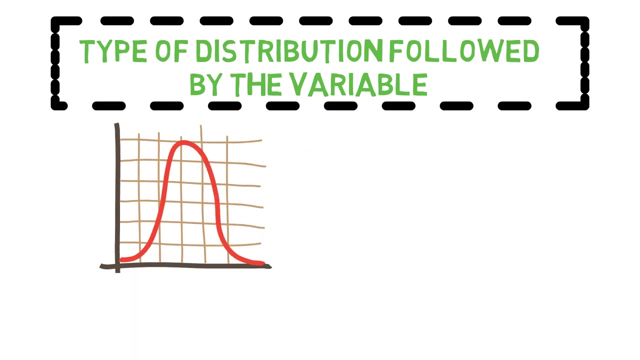 chi-square test. so I think you've got it, Bolu, okay. so now we come to the second factor, that is, type of distribution which is followed by the variable. whatever variable you want to study, you must check what kind of distribution it follows, like whether it follows a normal. 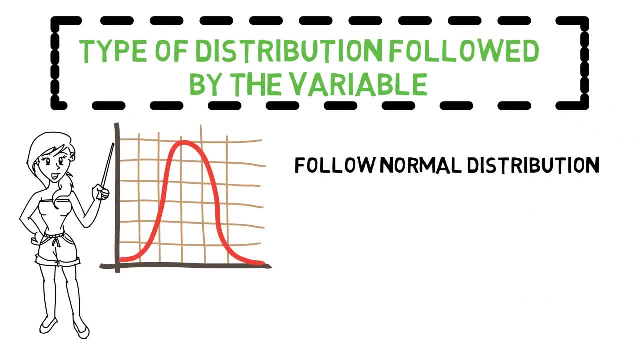 distribution like it is depicted by the red curve here, and whether the variable does not follow the normal distribution. in case it follows a normal distribution, you can go for parametric tests like ANOVA t-test, and in case if it does not follow the normal distribution, you can. 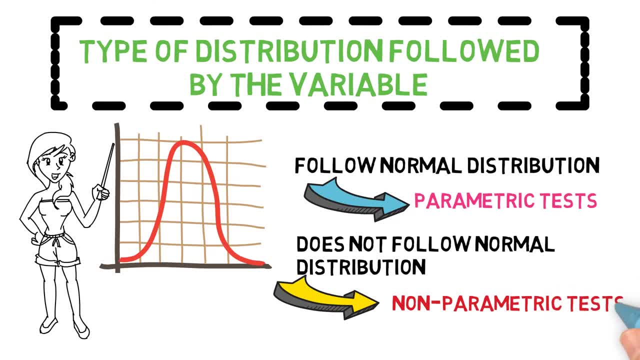 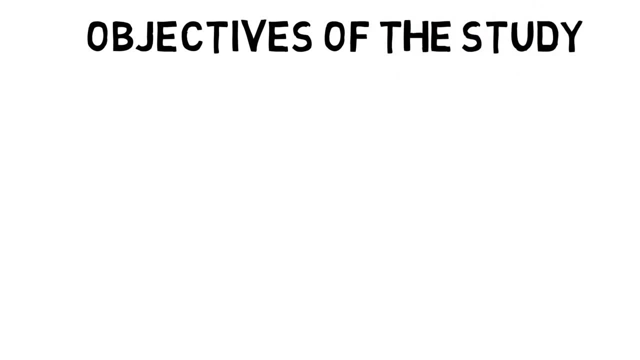 go for the non parametric test, then the next factor on which it depends is the objectives of the study. whatever objective you have in your study, it may be focused upon, like, say it, to test the hypothesis, and it's rather very simple that whenever you want to test any hypothesis, you can. 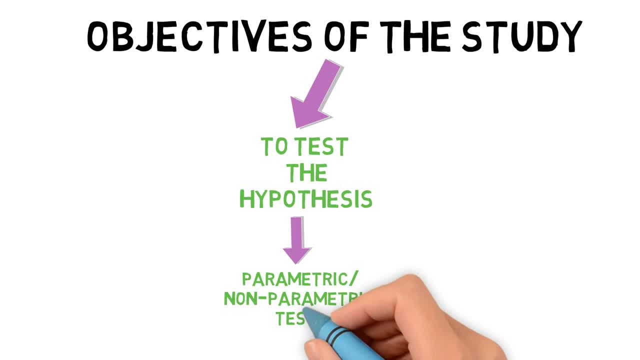 go for the parametric testings or for the non parametric testings or the tests, then on the other hand, your objective of the study may be to test a proposed model. suppose you have taken some variables and established certain relationships between those variables and now you want to check the relationships. so then you can apply, you can go for structural equation. 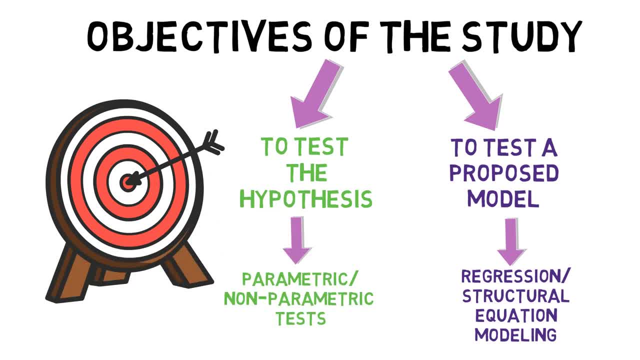 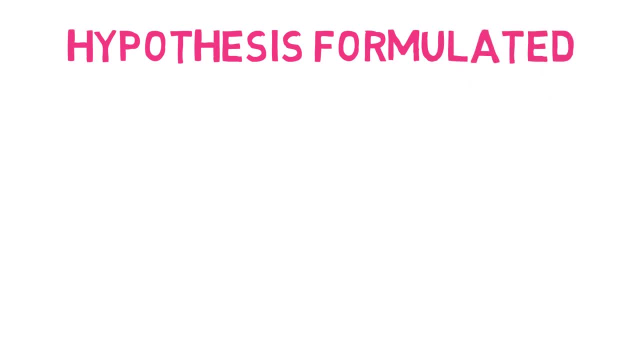 modeling or maybe regression analysis and so on. then we have the fourth factor, that is hypothesis formulated. so whatever hypothesis you make for your study, it can aim at. for example, it can aim at testing the association among the variables. so if you want to test the association, either you can go for Pearson correlation or you can go for the chi-square test. Now, on the other, 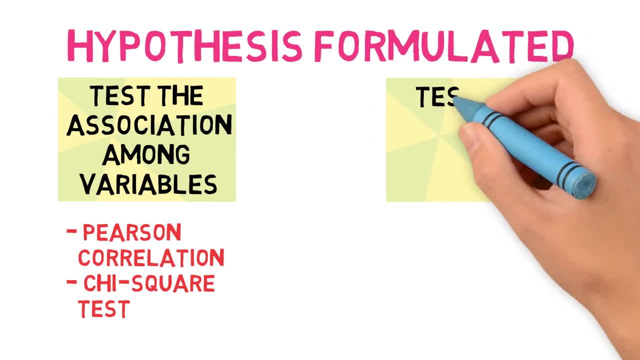 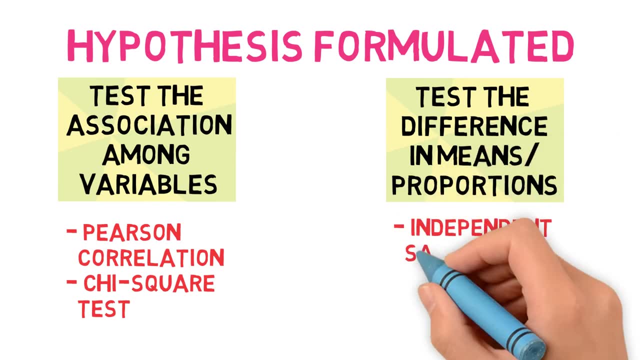 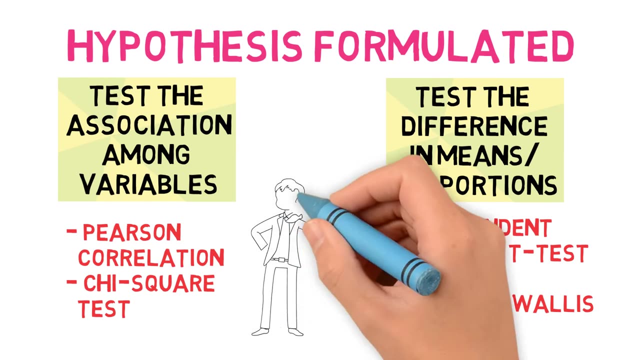 hand, suppose, if you want to test the relationship or the difference in the means or the proportions of the variables, So in that case you can go for independent samples, t-test or ANOVA, or you can go for the Kruskal-Wallis test and so on. So this was your fourth factor, and now we come to the fifth. 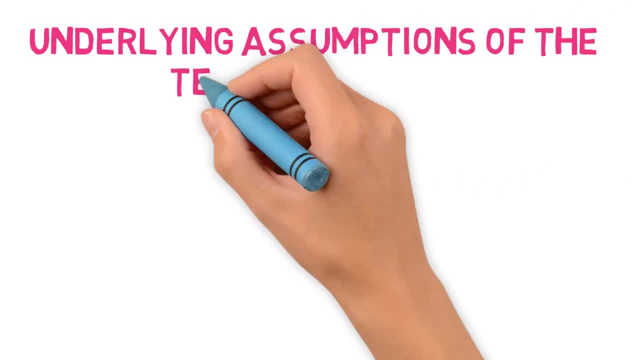 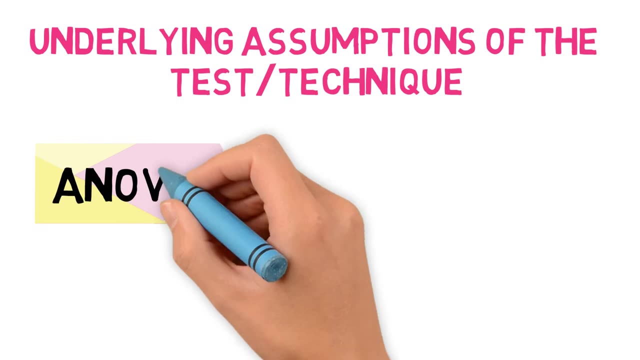 factor, that is, the underlying assumptions of the test or the technique you want to apply. Suppose you have checked all the situations and now you came on to the conclusion that, yes, I can apply ANOVA. So now, before applying ANOVA or analysis of variance, you need to check the assumptions.